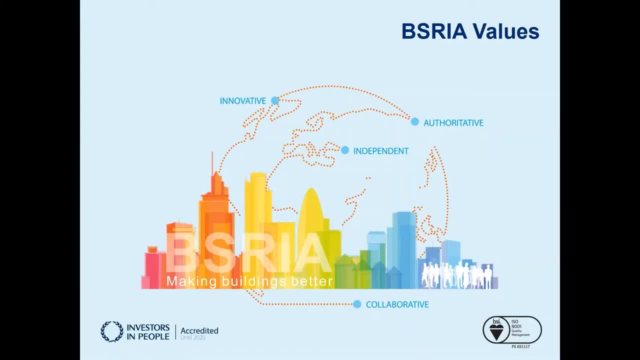 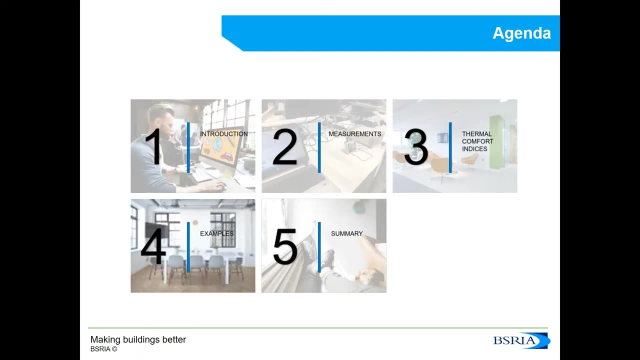 for free on the Bistria web. We're going to start today by introducing the concept of thermal comfort And then we're going to continue with the measurements and instrumentation that we have to take to measure thermal comfort. We're going to talk about the results of thermal 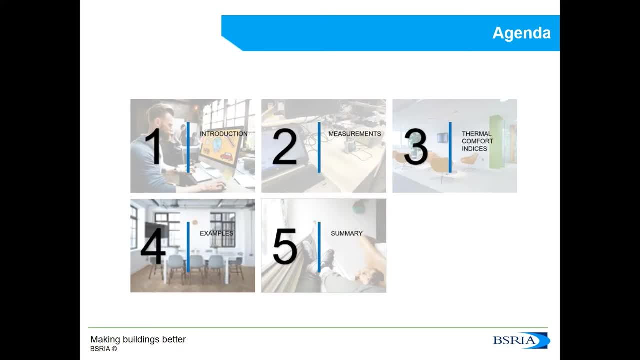 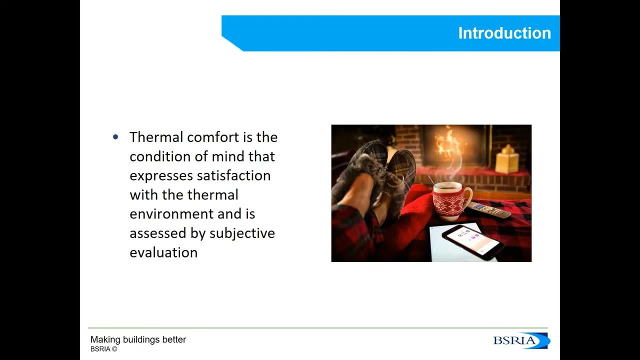 comfort or the thermal comfort indices. And then I'm going to show you some examples where Bistria has calculated thermal comfort. And finally, we're going to sum up this presentation. So, to start, we're going to give a brief introduction of what thermal comfort is. Thermal comfort. 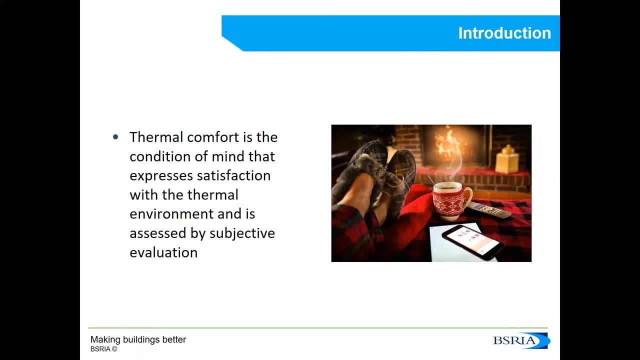 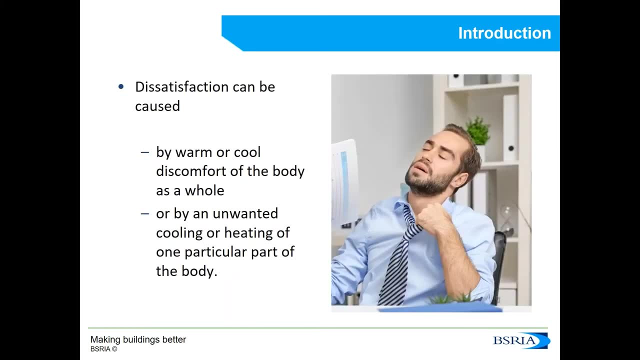 is the condition of mind that expresses satisfaction with the thermal environment and is assessed by subjective evaluation. Dissatisfaction with the environment can be caused by feeling too hot or too cold, if we take into consideration the whole of the body, or also by having the feeling of cooling. 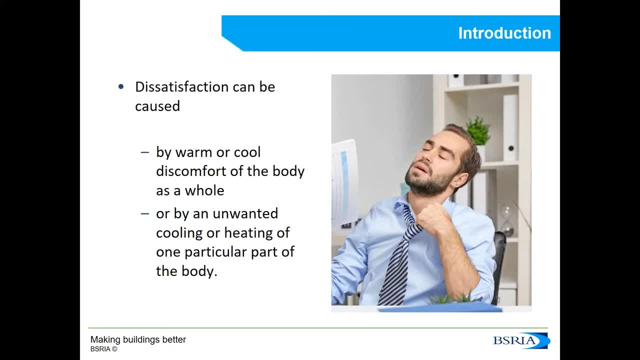 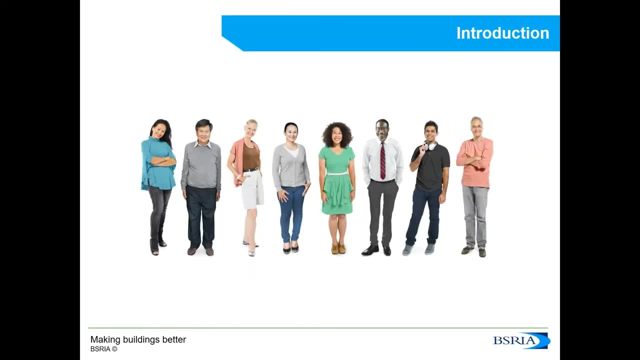 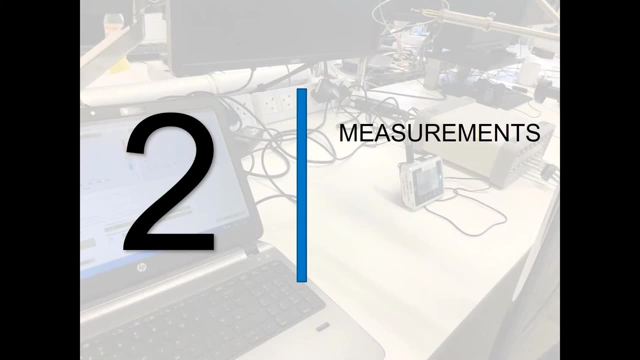 or heating in the body, In a particular part of the body, which is known as local discomfort. Due to individual differences, it is impossible to specify a thermal environment that will satisfy everybody. In the next section we're going to see how to measure thermal comfort. There are two. 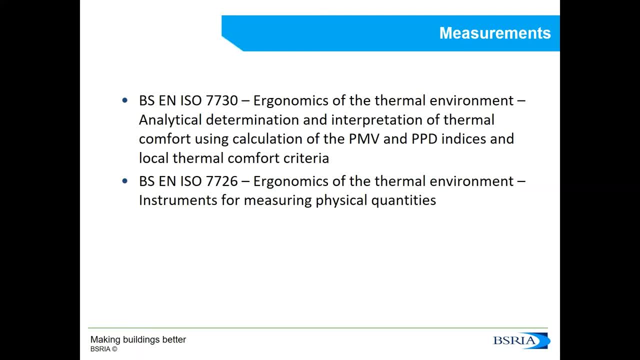 standards that relate to thermal comfort, and they are both based on the work that Professor Olle Fanger from the University of the United States has done, And they are both based on the work that Professor Olle Fanger from the University of the United States has done. 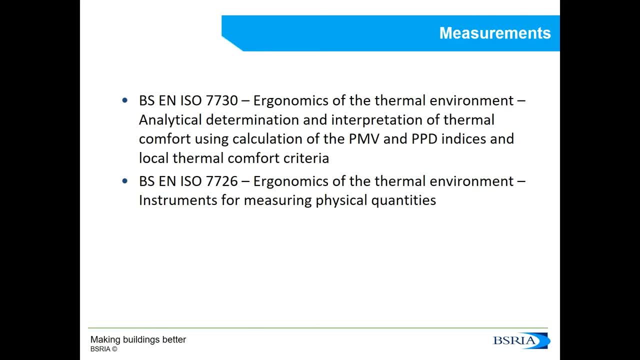 They are both based on the work that Professor Olle Fanger from the University of the United States has done. He conducted an experiment in Germany. He conducted an experiment in Germany. He investigated thermal comfort and he experimented his results with a very large number of volunteers, and the standards were developed. 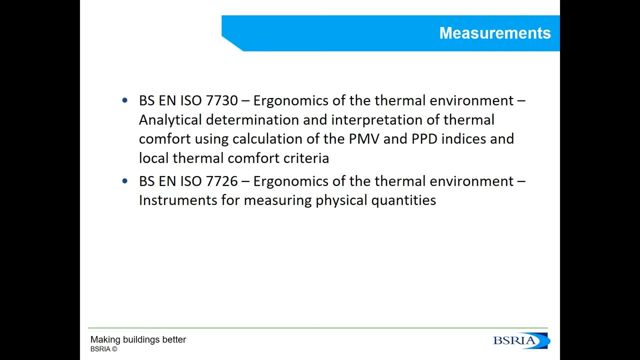 So the first standard you can see here is BS EN ISO7730.. And this one explains the calculation of thermal comfort and the standard 7726 deals with instrumentation. So the standard 7726 deals with instrumentation And this one explains the calculation of thermal comfort. 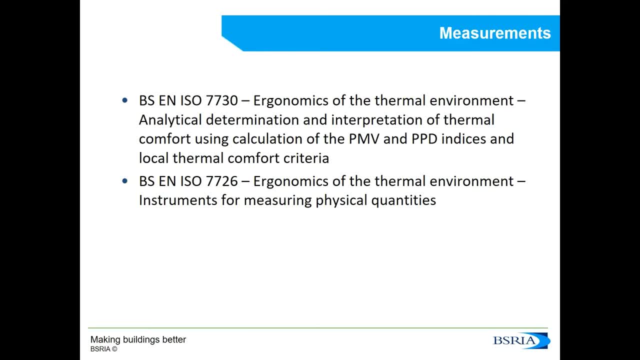 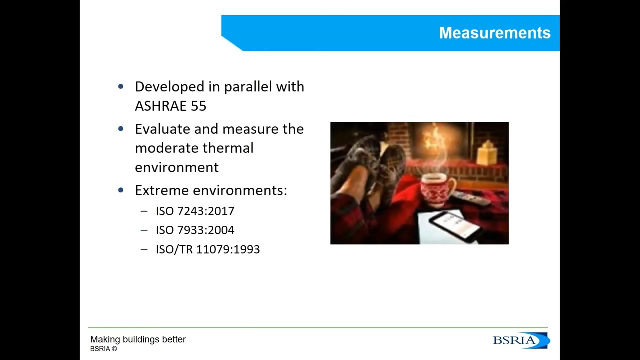 and the calculation of the different temperatures and humidity and air velocity and instrumentation that you have to use. These are the two standards that we normally use at Visria, but also ASHRAE 55 is another standard based on thermal comfort. Both standards were developed in parallel. 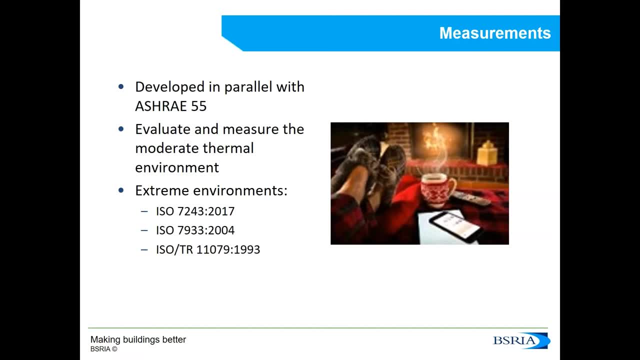 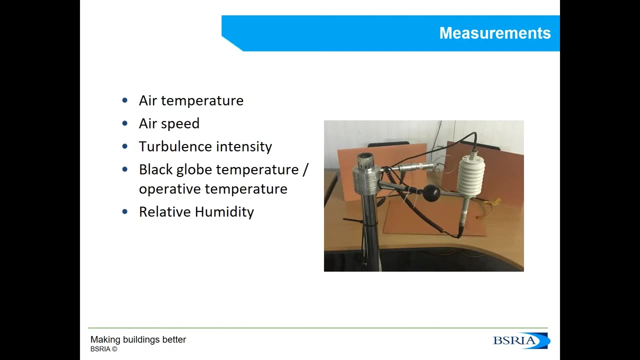 and they refer to the moderate environment. There are also other standards that deal with extreme cold or extreme hot environments, if you need more information on those. To measure thermal comfort involves a little bit more than measuring the temperature and measuring the humidity, although these are two parameters that we have to measure The 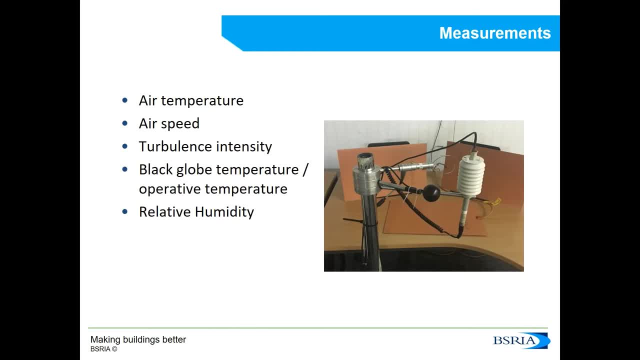 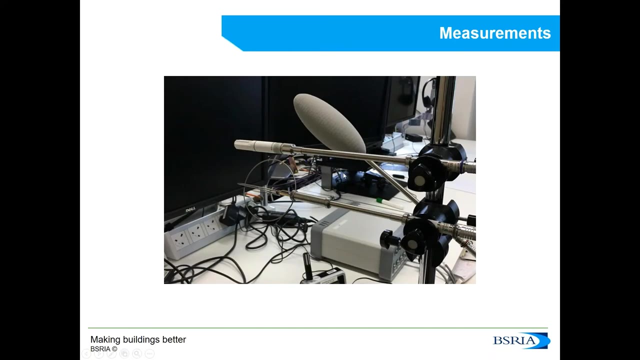 other parameters that we have to measure are the temperature, the air speed and the temperature temperature, the turbulence intensity and the globe temperature, as you can see here using a black globe. If you're not measuring the black globe temperature, you can measure. 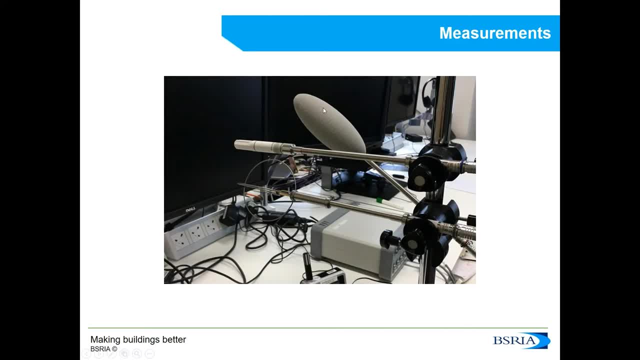 the operative temperature using this sensor that looks like a microphone. instead, You have to apply slightly different calculations, but you can still obtain the thermal comfort indices. What you can see here, also in white, is the humidity sensor. What you can see here is an anemometer that has a shield, a metal shield, and this is 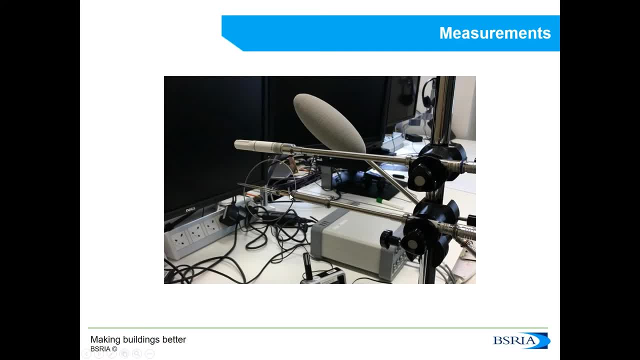 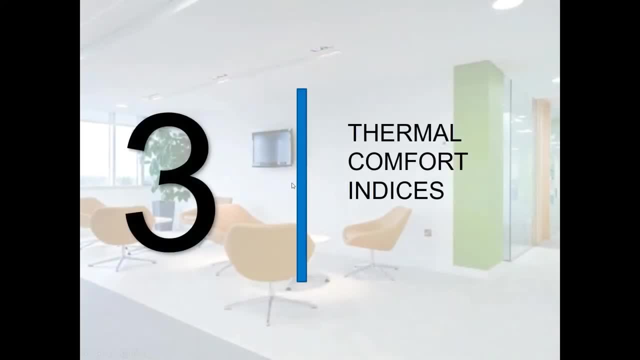 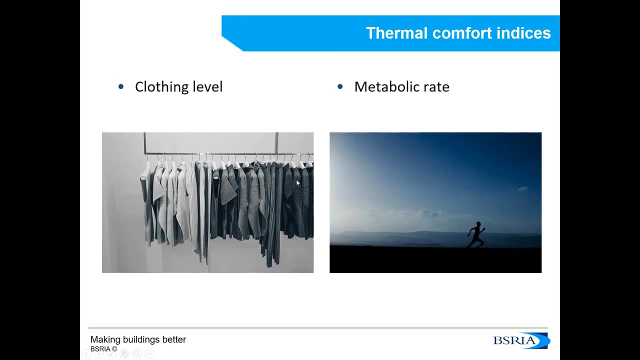 just to protect the anemometer. This anemometer measures the air temperature and the air speed as well. Before I start talking about the thermal comfort indices, I would like to mention that, in order to calculate thermal comfort, we have to take into consideration the clothes that 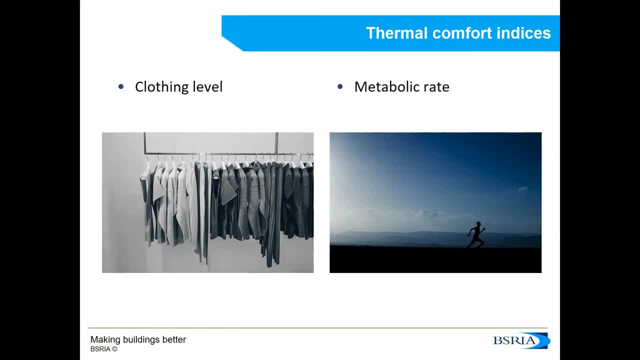 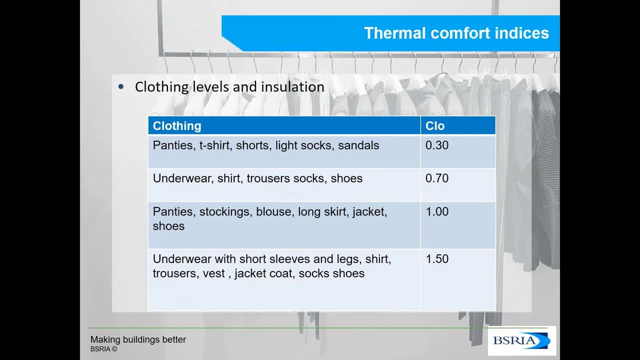 a person is going to wear and also the metabolic rate. To start with the clothes, we have to take into consideration very important things that include thermal insulation. Of course, we don't feel the same. Episode 20: The Emotional Temperature. Calculation of theאת. binder temperature and temperature with an environment where winter clothes are. 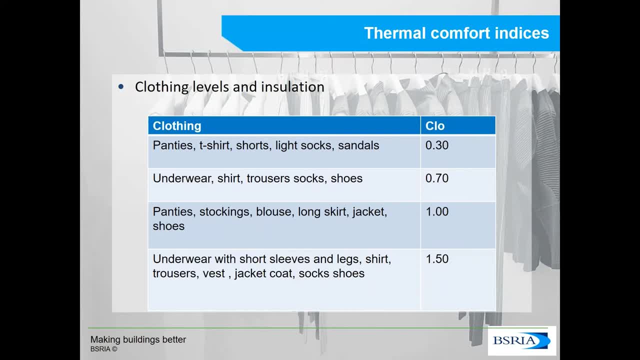 made up of hatgirl beaucoup gloves or scarf. Their general touch of home wear and home bath is apple. And there is also a list of individual clothing components, so if you cannot find exactly what the design is for you can always add up the clothing levels for each component individually. 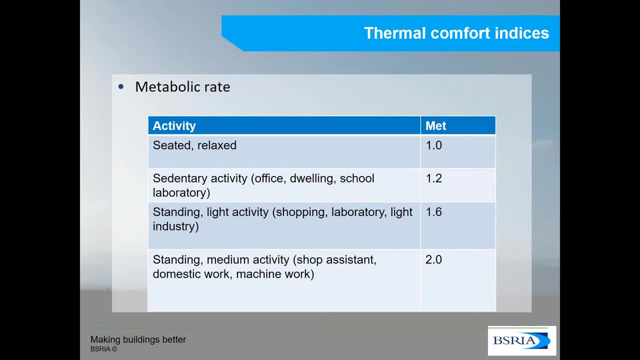 And the next thing to take into consideration before calculating the thermal comfort indices is the metabolic rate. So the metabolic rate gives us an indication of the activity that we are carrying out and, as you can imagine, a person will not feel the same in the same. 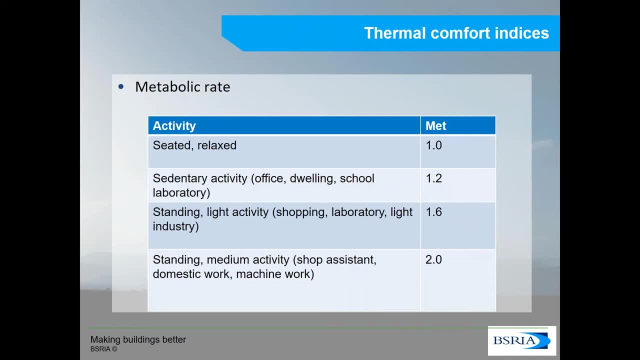 environment if, for example, they are sitting down or if they are running. So in an office environment we probably would have a metabolic rate of 1.0 or 1.2, which is equivalent to a sedentary activity, because in an office we're not normally getting up and down and walking around. 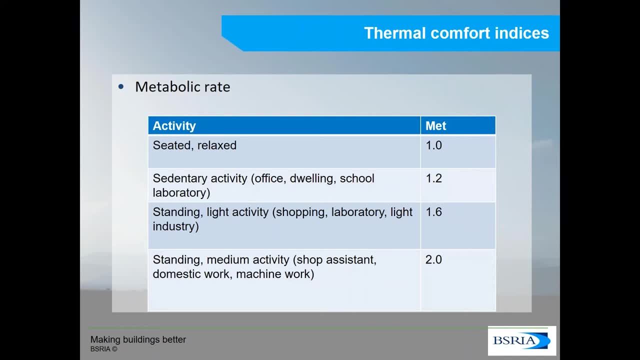 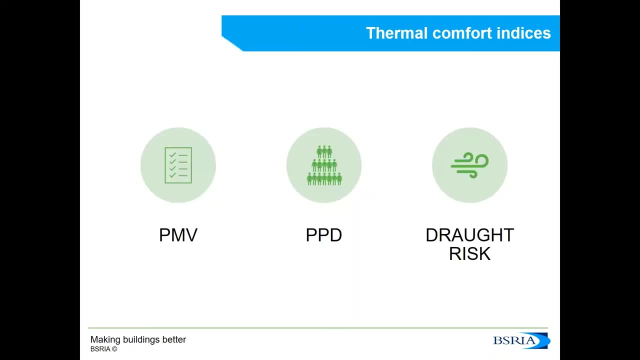 the office But, for example, in a hospital environment, we could have a higher metabolic rate. So once we take into account the air speed, the air temperature, the humidity, the metabolic rate, the clothing levels, the globe temperature, we can calculate the thermal comfort indices, which are: 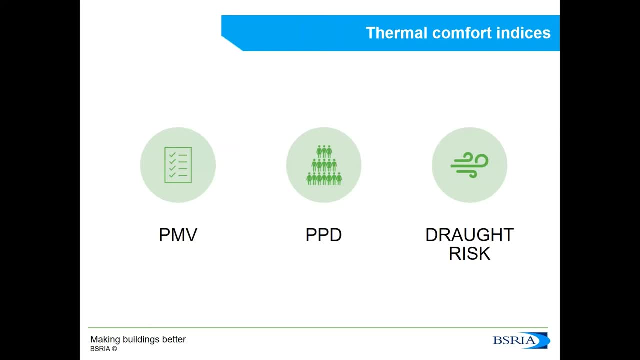 PMV, or predicted mean vote, PPD, or predicted percentage of dissatisfied, and draft risk- normally A few more. that we'll see at the end of this presentation. So to begin with the PMV, what we have here is the thermal sensation scale, So the thermal 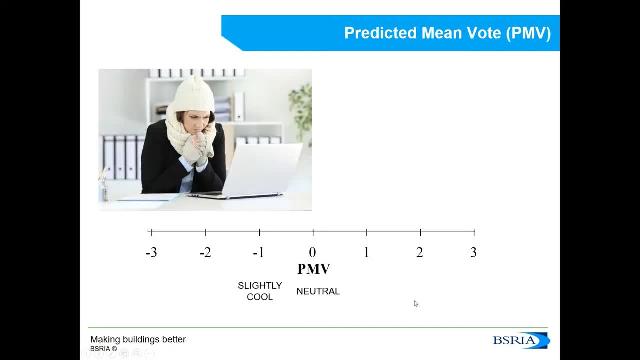 sensation scale is a scale of minus three to plus three, in which zero means that a person would feel neutral with the environment. minus one would mean that they feel slightly cool. minus two would mean that they feel cool. minus three would mean that they. 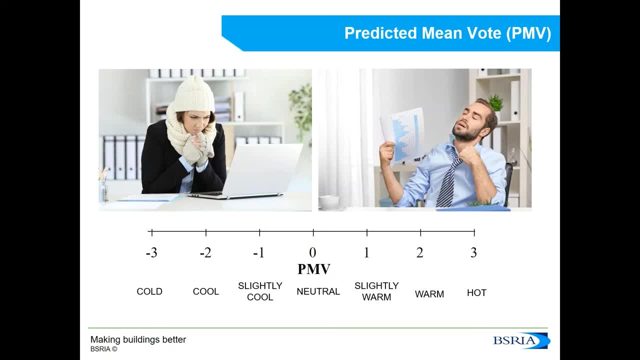 feel cold And then, on the other side of the scale, we would have one, two and three for feeling slightly warm with that environment, warm or hot with that environment. So if we asked a lot of people how they feel in an environment and to vote on this scale, 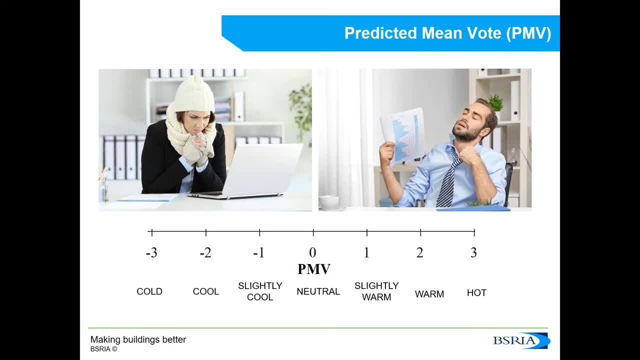 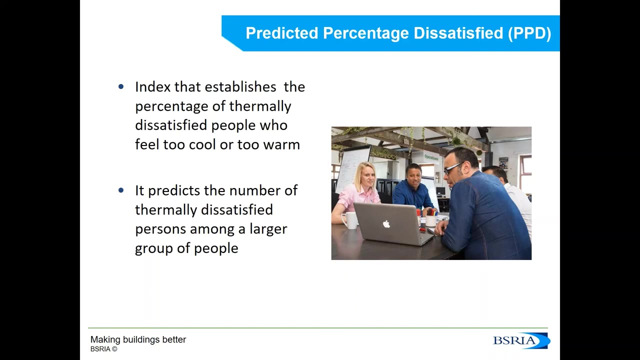 and we calculated the average. that would be the mean vote, And the predicted bit is because we do not ask people, but we predict how they are going to feel advance. The next index I'm going to talk about is the PPD, or the predicted. 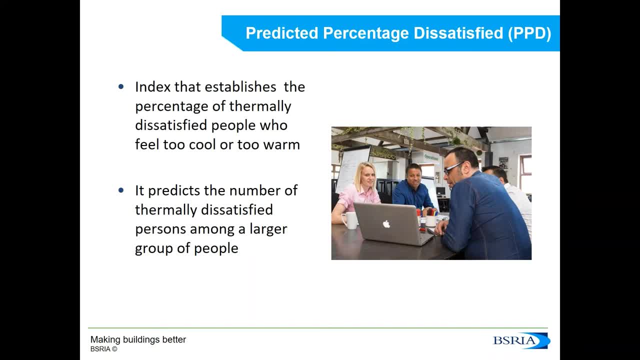 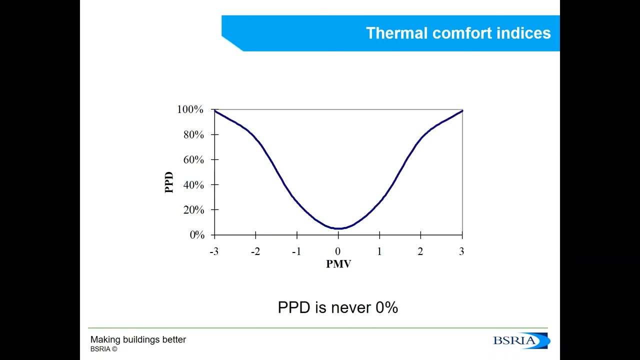 percentage of dissatisfied and, as its name indicates, the PPD predicts the number of people who are going to feel uncomfortable in a certain environment And, as we can see here in this graph, PMV and PPD are related. so if people voted, 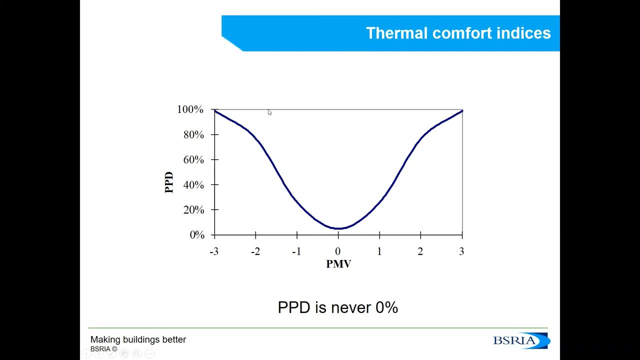 that they were feeling extremely hot in an environment or very cold in an environment. then a hundred percent of people would feel dissatisfied with this environment. so it would be perhaps better to go back to design stage, for example, and review your design so that people would feel more. 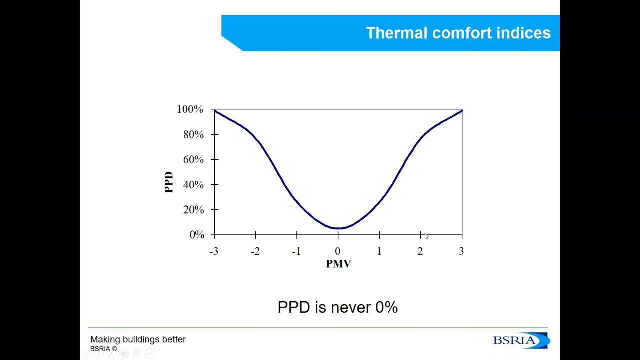 comfortable with the environment And as the PMV approach is zero, then we see that the PPD goes down. But if you notice, here, PPD is never zero percent because there's always going to be a percentage of people who feel dissatisfied with the. 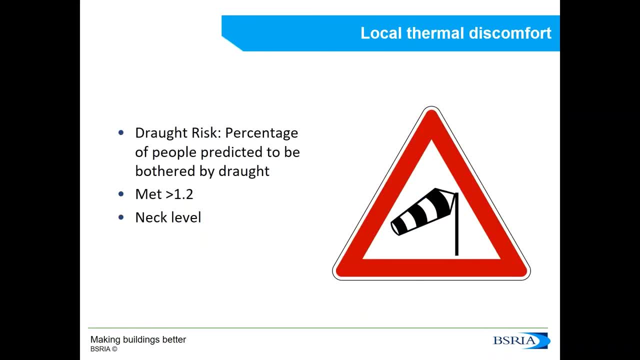 environment. As I mentioned before, we can feel satisfied or unsatisfied with the environment, taking into consideration the body as a whole, and this is where the thermal comfort indices of PMV and PPD are important- but we can also have local discomfort, for example. 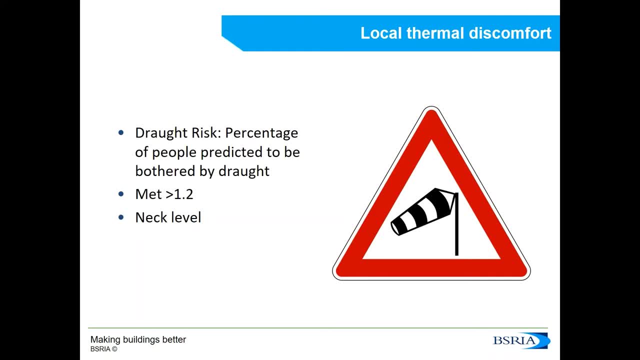 if we feel a cold draft of air blowing down our neck, for example, because we are in the proximity of two supply grills that are clashing with each other and they are just dumping air on our neck. So the draft risk calculates the percentage of people who 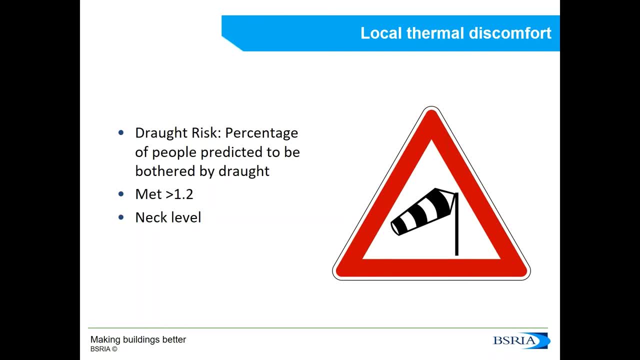 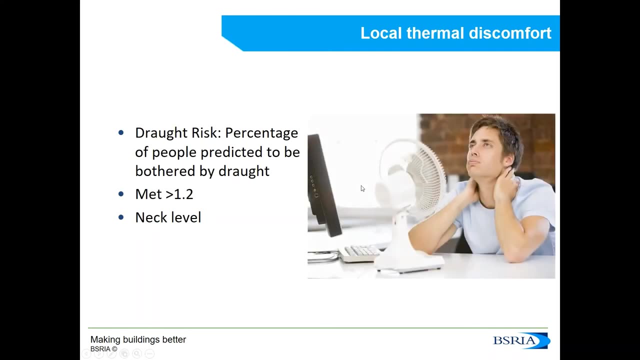 are likely to be bothered by a draft, and this is normally when our level of activity or metabolic rate is less than 1.2, and is normally felt at neck level. The reason why we talk about draft risk when the metabolic rate is less than 1.2 is because 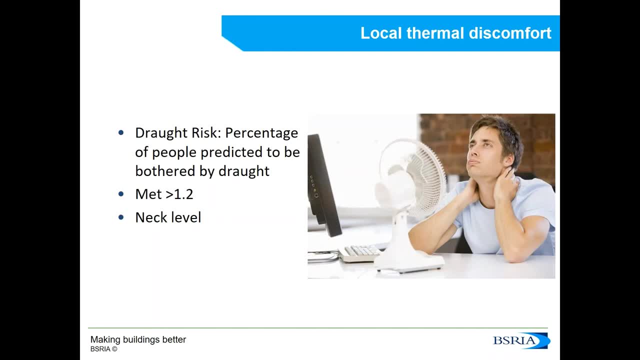 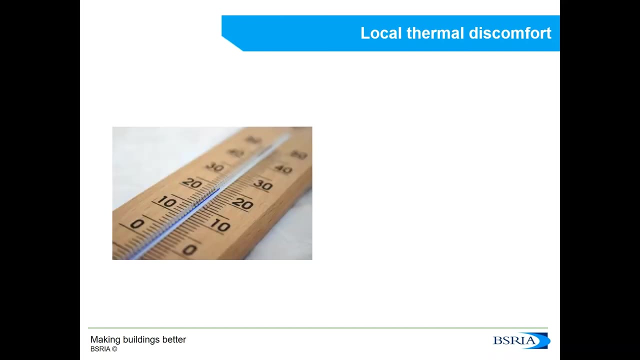 if you imagine the following situation: if we are in a very hot office or we are doing a lot of work and we put on a fan, we would certainly be feeling a draft, but we will probably find that quite comfortable. Right In here we can see other reasons. 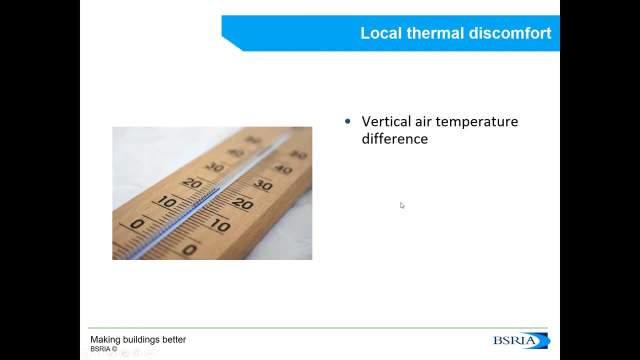 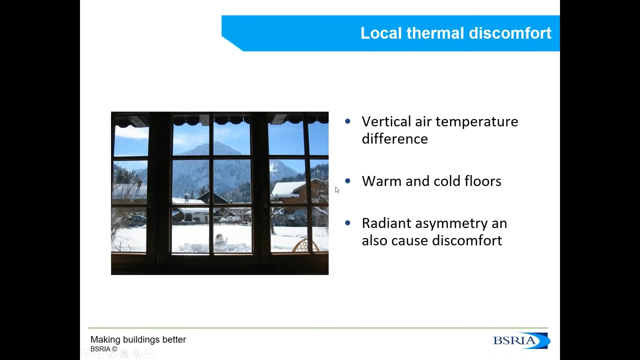 why we can feel uncomfortable with the environment, which are actually having a large vertical air temperature difference. warm and cold floors can make us feel local discomfort and also radiant asymmetry can cause discomfort. Radiant asymmetry is what we experience, for example, when we are close to a fire. we would feel very hot on one side and relatively colder. 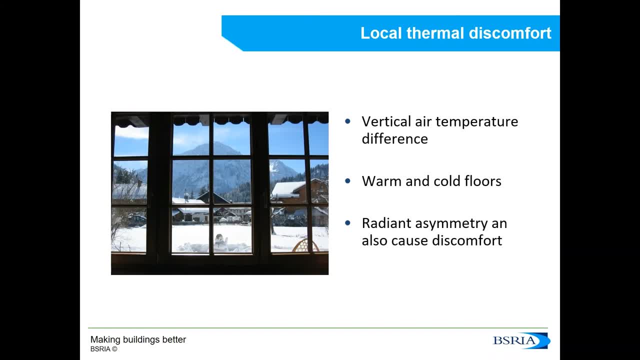 on the other side Or when we are close to a cold window. So if there is an abnormally high temperature difference between the head and ankles- up to eight degrees- there is a percentage of people who are also going to feel uncomfortable And, as I mentioned before, it affects more. 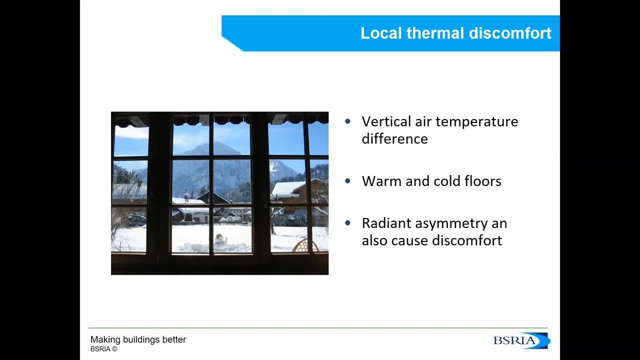 people who are at a light sedentary activity, And if the floor is too warm or too cold, the occupants could feel uncomfortable. And for people wearing light indoor shoes, it is the temperature of the floor rather than the material of the floor which is important for comfort. 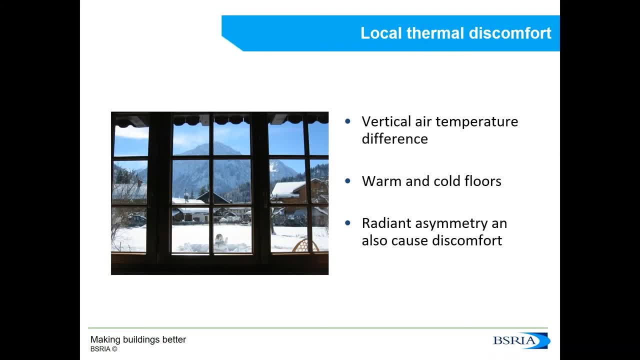 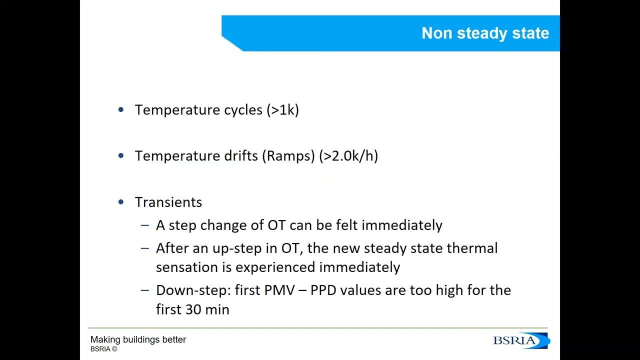 And finally on radiant asymmetry, which can also cause discomfort. people are most sensitive to radiant asymmetry caused by four aspects, which could be warm ceilings, cold ceilings, cold walls or warm walls. So the standard establishes formulas to calculate a predicted of the satisfied based on these. 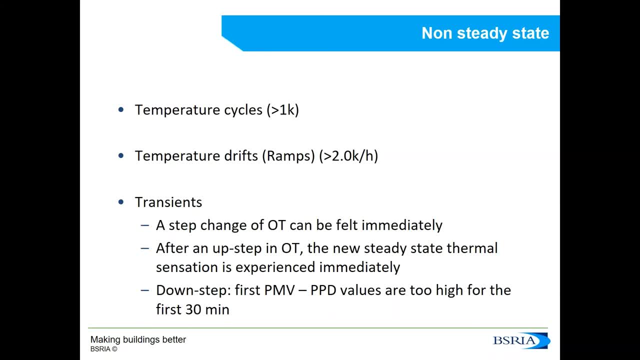 factors of local comfort. But these calculations that we have gone through they refer to steady state conditions. But in a real building there are temperature variations due to, for example, the influence, the controls, for example. So, for example, the temperature of the building, the temperature. 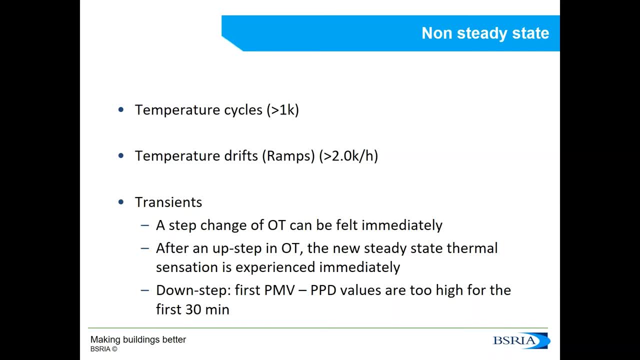 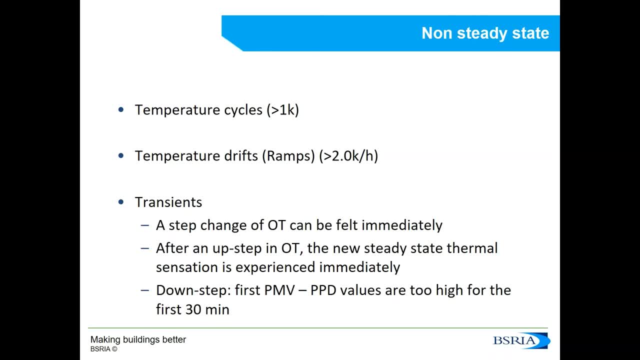 temperature drifts or ramps and transients, So temperature cycles can occur due to the control of temperature in space, And if the peak variation is less than one degree, the recommendations and the calculations that we have seen for thermal comfort can be used. 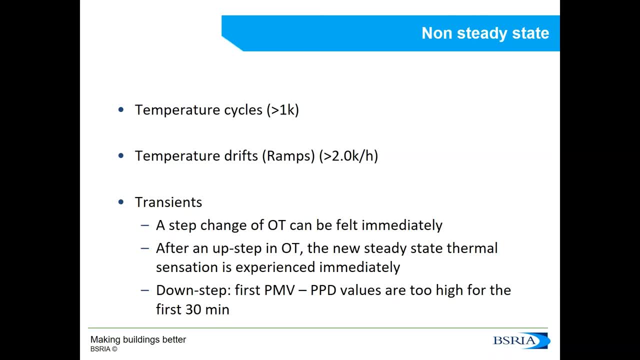 And then with temperature drifts or ramps if the rate of temperature changes for lower than two degrees per hour. we can still use these methods. And regarding transients, well, in general, the following statements can be made. So a step change in the operative temperature. 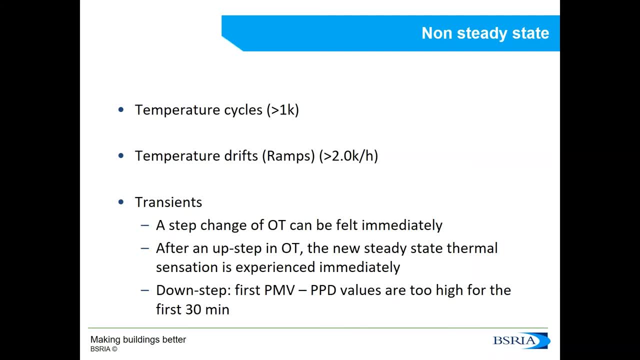 can be felt instantaneously and after an upstep in the operative temperature the new steady state thermal sensation is experienced immediately. But following a downstep in the operative temperature, the PMV and PPD values that we're going to measure are probably going to be. 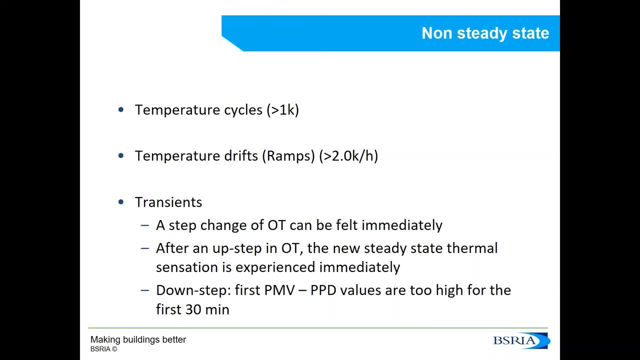 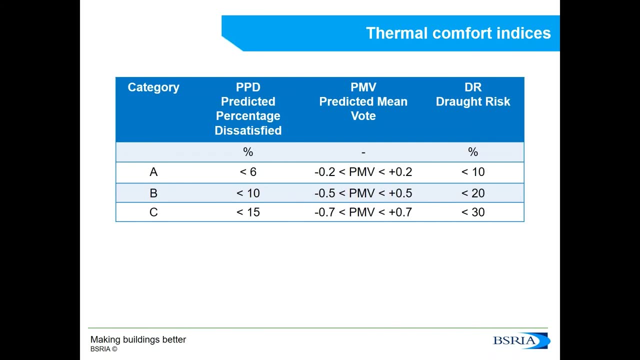 too high for the next 30 minutes until we acclimatise ourselves to the new thermal conditions. And finally, what we can see here is: in the standard, there is a classification of the thermal comfort results into three categories: A, B or C, based on the results of the PPD, PMV and draft risk. And even though 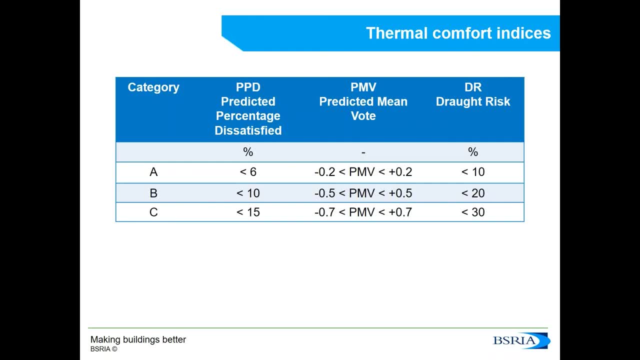 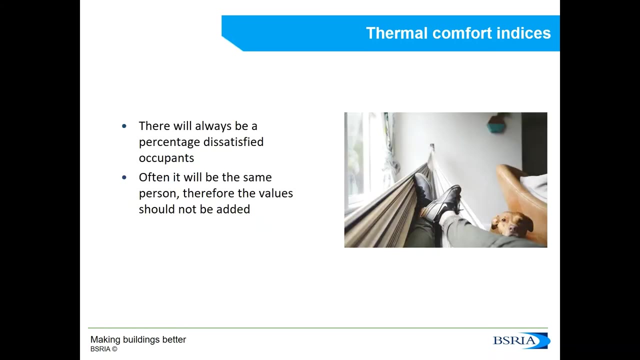 this is not compulsory. this table, for example, could be used at contractual level, So the signs would have to meet the requirements A or B or C of this table, for example. And finally, just note that there will always be a percentage of dissatisfied occupants. 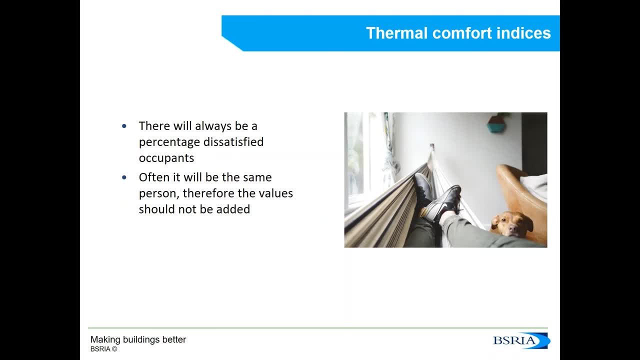 but it's possible to specify environments that are going to be acceptable for a large percentage of the occupants, And it's often the same person who would be sensitive to different types of local discomfort. So, for instance, a person sensitive to draft may be also sensitive to local cooling caused by radiant asymmetry or by a temperature of. 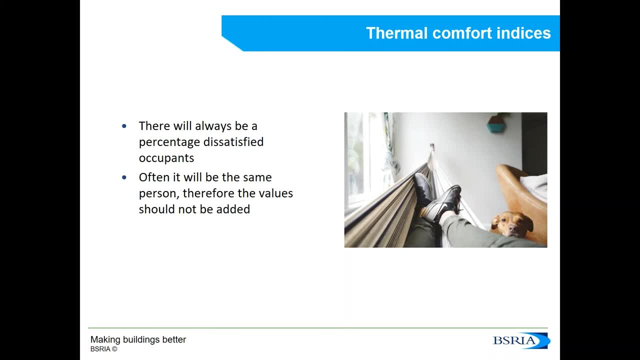 the temperature. So the results are very similar And the results are very similar. So the results are very similar And the results are very similar And the results are very similar. This is why the percentage of dissatisfied occupants that we have calculated before 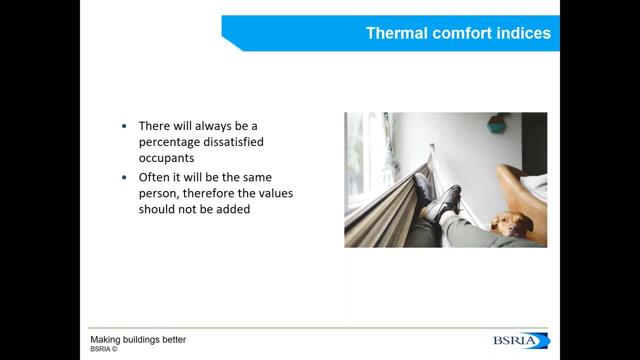 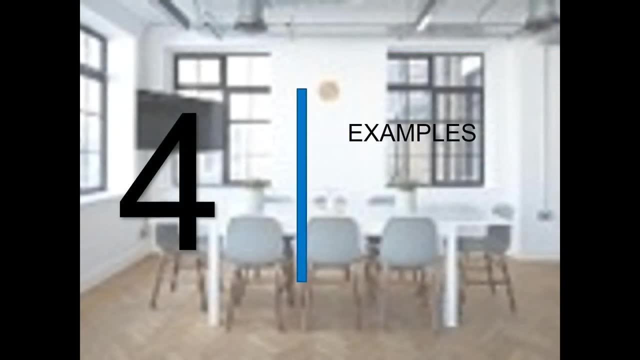 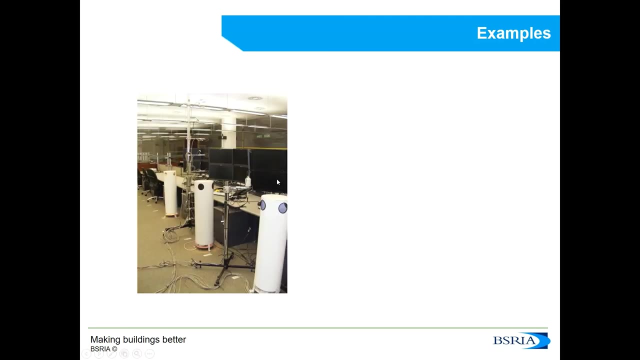 should not be added because normally they will be referring to the same person, Right? So here we have some examples. Well, we have to measure thermal comfort at Base Rehab. We normally calculate the thermal comfort indices in mockups Before we use BASER. we 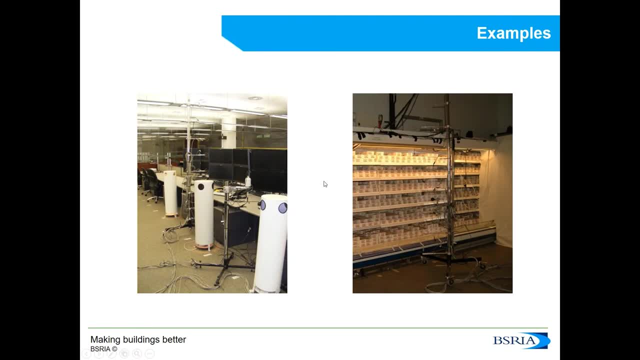 will use this before a building is actually built, or we can go. we can go on site. so, as we see here on the left hand side, we were measuring the thermal comfort in in a building that had a high, quite a high, quite a high heat load, because each 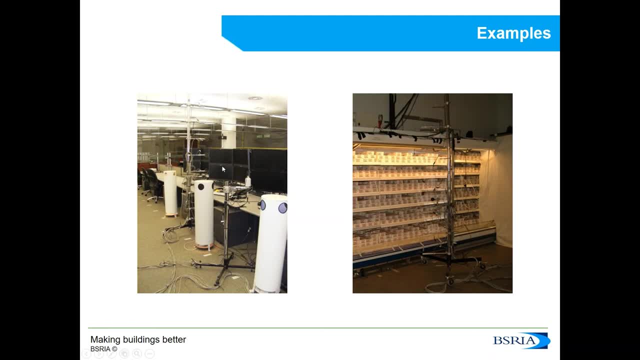 person was using a very large amount of computers and screens and on the left hand side- on the right hand side- we can see a study that we did on on the thermal comfort in the supermarket aisle. so we were measuring other things rather than the thermal comfort only, and we were also measuring the, the duty of the. 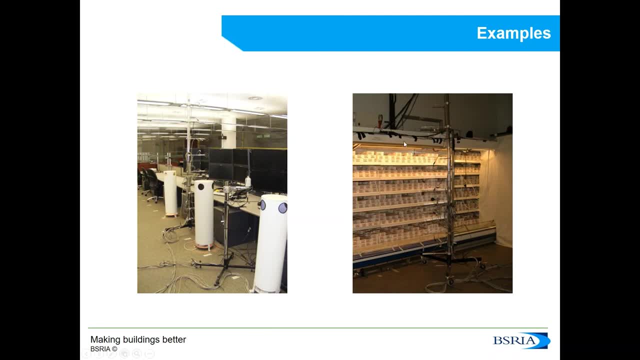 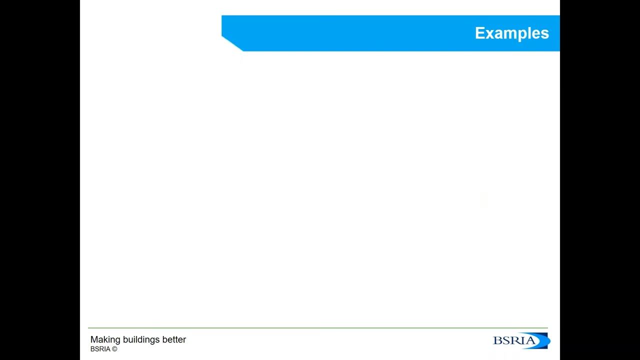 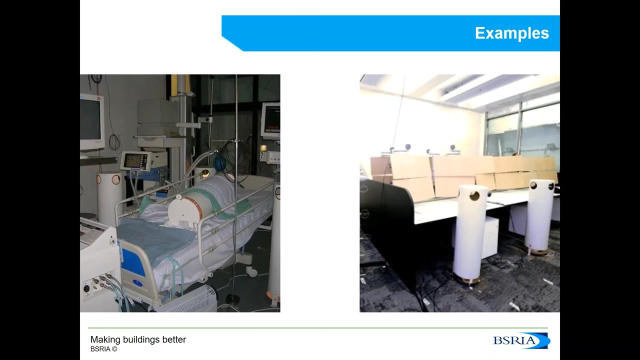 of the refrigerators and the temperature of the product, but we were also measuring the thermal comfort of several, several people, either working away from these people or actually visiting- maybe workers or visitors- to the supermarket. and in here you can see other two examples in which we also measure the thermal. 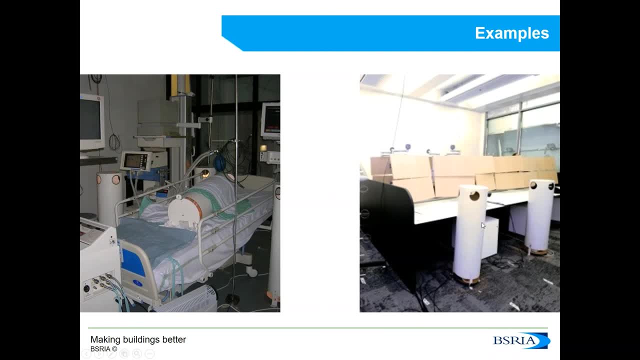 comfort. this was a mock-up for an office building in which we measured thermal comfort of different ventilation systems and, on the left hand, control of the staff and the patients, and was also doing other tests on pressure differentials, on the pressure stabilizers and on infection. 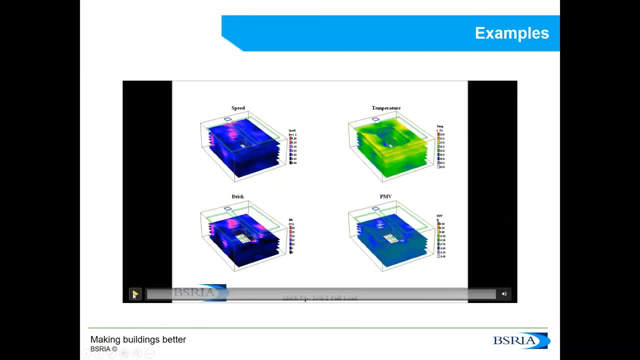 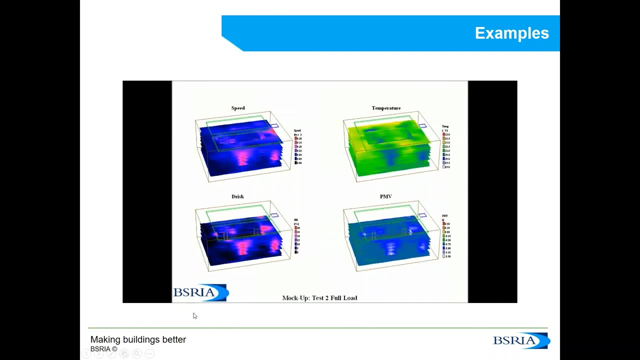 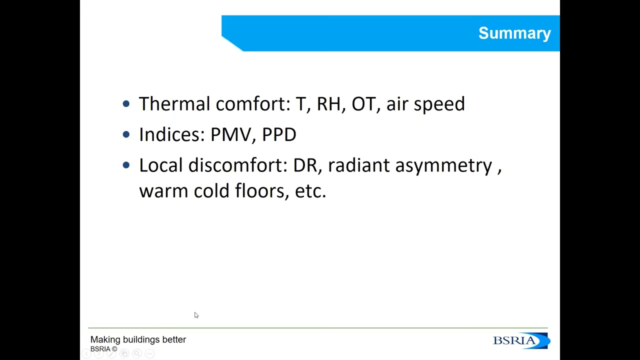 transmission, and here you can see an example of the results. so, to finalize this presentation, we have seen how, in order to measure air behaved with賦 siériecomfort, we have to take into consideration the temperature of the air, the speed of the air, the relative humidity, the operative temperature or 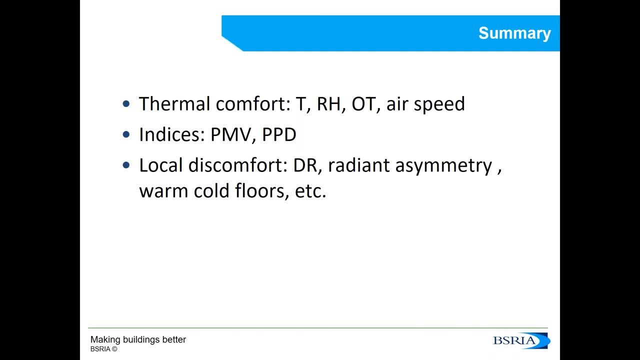 the가 Paust import on presenting high temperature and we the air and the relative humidity, the operative temperature, our clock temperature. we have seen how to calculate the thermal comfort indices of PM, v and P PD. we also have to take into consideration the, the air and the relative humidity, the operative temperature or the clock temperature. we have seen how to do in practice. in factuum a young man suffer niece have to take into consideration the click. we also have to take into consideration the four the频. here's a bit a series. speaker house: very meteoric, comfortable, get ready for. take care in the purely isn't quite things that we have. you 37 black put on the, suppose youerie that guy get right. our next physical devices: you have the.